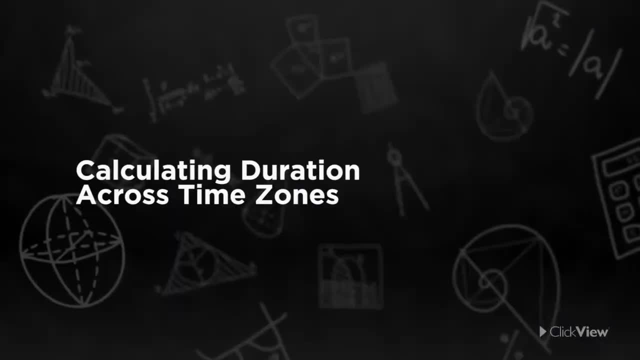 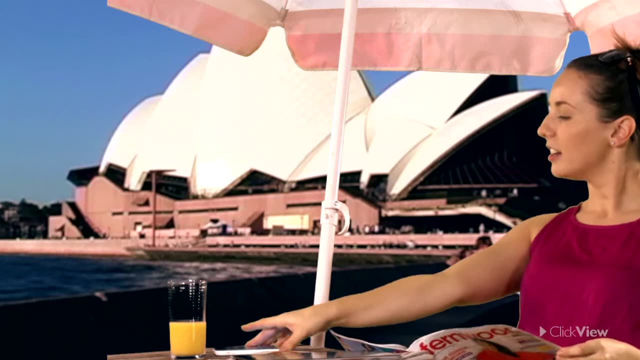 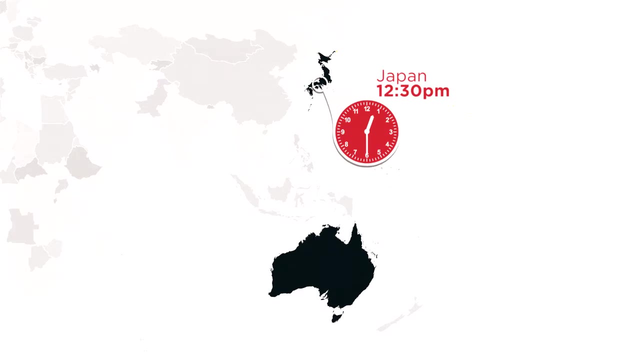 Hey, I'm chatting with my friend in Japan. She's having her lunch right now. It's 12.30pm. I live here in Sydney where it's 1.30pm. I've had my lunch already. Japan is in a different time zone to the eastern states of Australia. 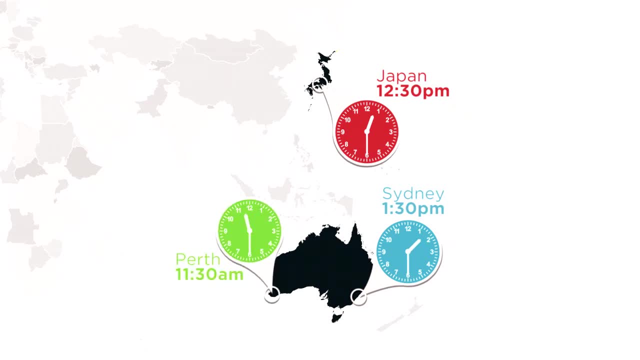 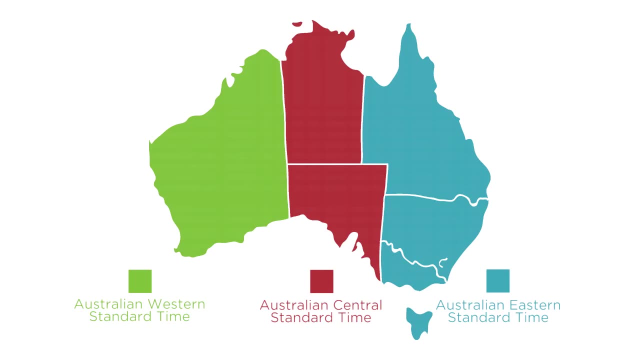 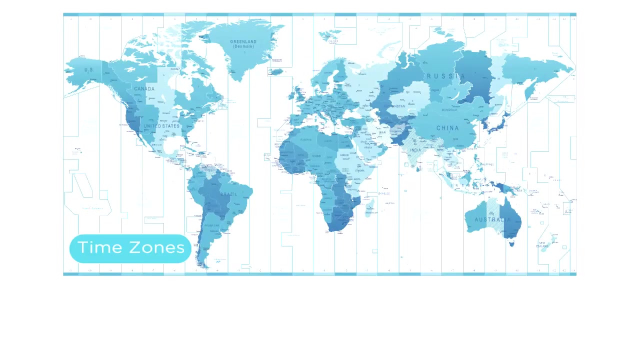 Over in Perth. it's 11.30am now, so Japan is in a different time zone from Perth as well. Australia is a large enough country to have more than one time zone. In fact, it's got three. The time zone in any place around the world depends on its longitudinal location. 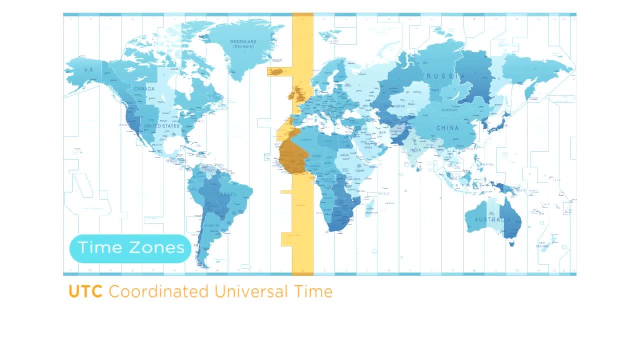 The reference point is known as UTC or Coordinated Universal Time. It's sometimes called Greenwich Mean Time or GMT. Australia and many parts of Asia are between 8 and 10 hours ahead of UTC. Cool, My friend says she's coming over to Sydney next holidays. 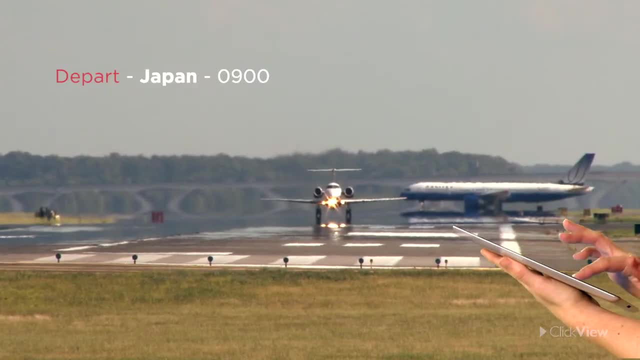 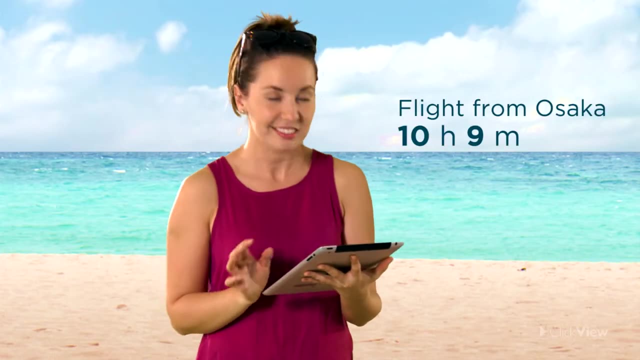 She's booked her ticket already. She flies at 0900 hours or 9am on a Wednesday. Let me see How long does the flight from Osaka take? OK, So what time will she land if there are no delays? 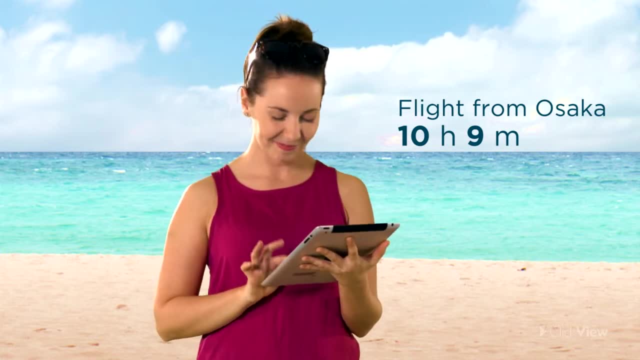 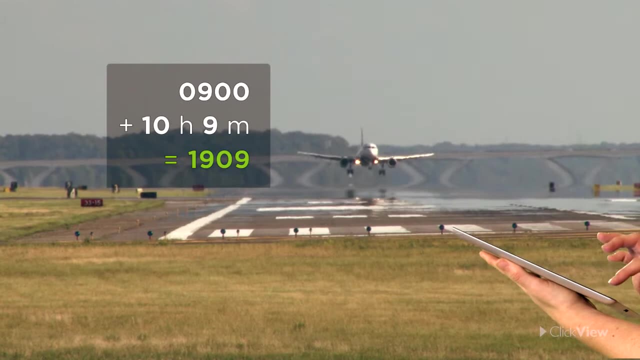 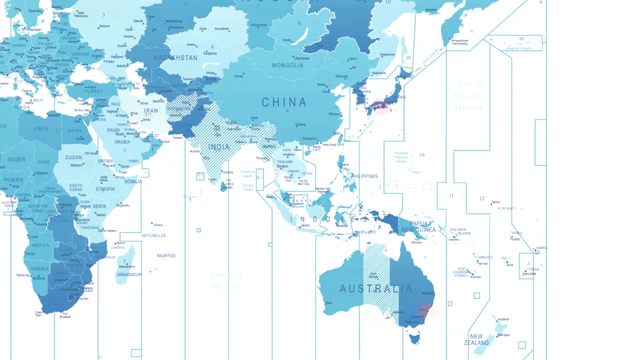 I can work that out using a simple equation: 0900 plus 10 hours and 9 minutes equals 1900, 09 hours on Wednesday. Uh-oh, Wait a minute. Sydney and Osaka are in different time zones, remember. 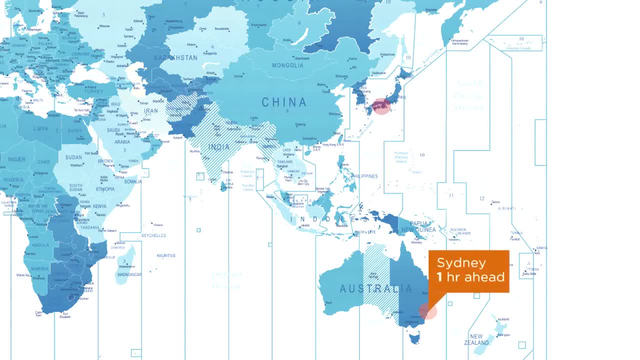 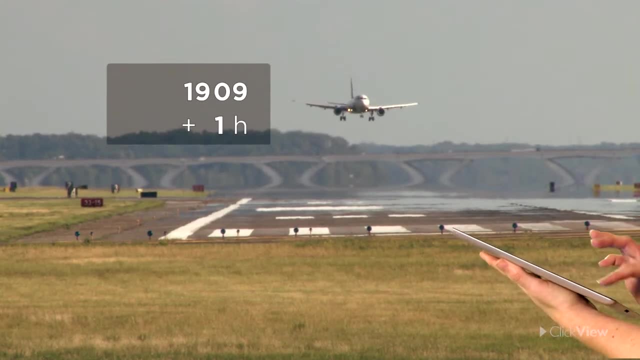 So Sydney is one hour ahead of anywhere in Japan. So it's 1900: 09 hours on Wednesday. So it's 1900: 09 hours plus one hour. She'll be landing at 200: 09 hours in Sydney. That's expressed in 24 hour time. 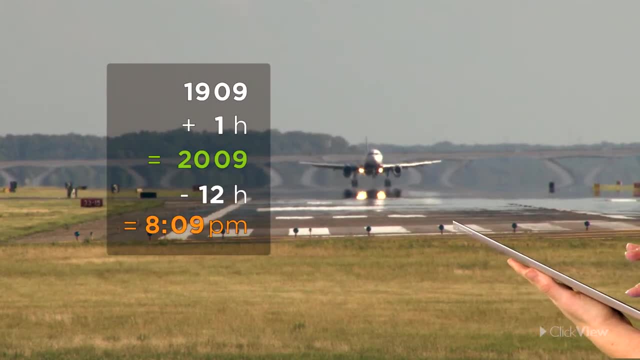 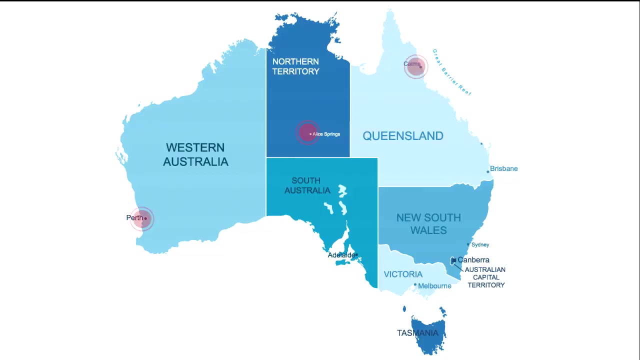 So in 12 hour time it will be 9 minutes past 8 in the evening, Or 8.09pm on Wednesday evening. She sent me her whole itinerary. She's also visiting Cairns, Alice Springs and Perth while she's here. 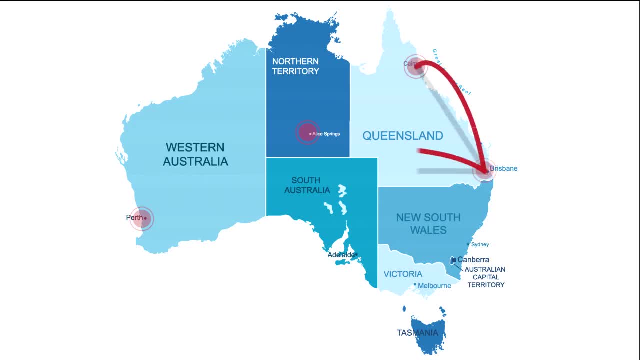 She's flying overnight from Cairns to Perth via Brisbane. She leaves Cairns at 11.45pm and lands in Brisbane, which is the same time zone as Cairns, at 5 minutes past 2am. So how long is that flight? 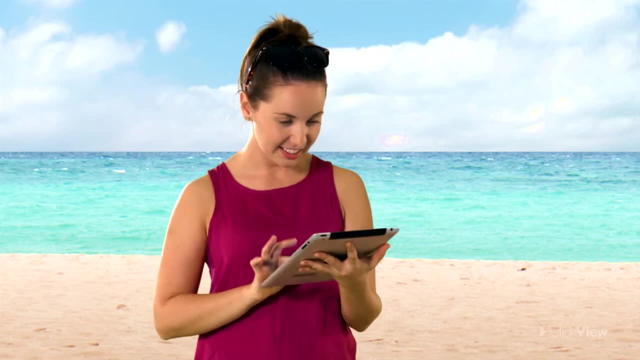 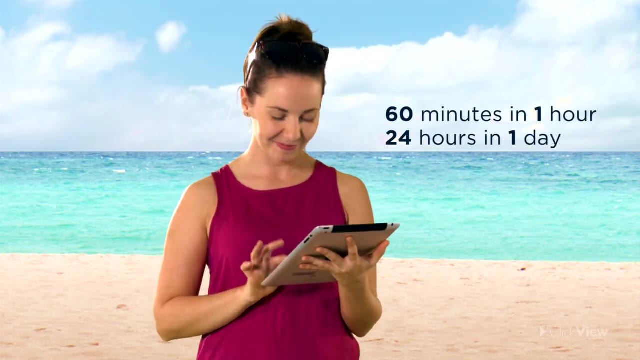 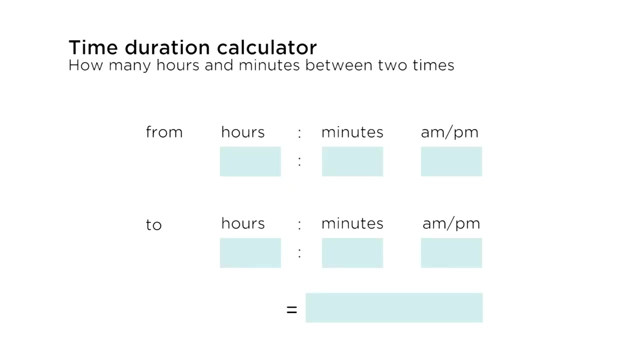 Calculating times like this can get a bit tricky because we're not using numbers to the base 10.. There are 60 minutes in an hour And 24 hours in a day, So I'm going to use my online time calculator. OK, it's 11.45pm, then 2.05am. 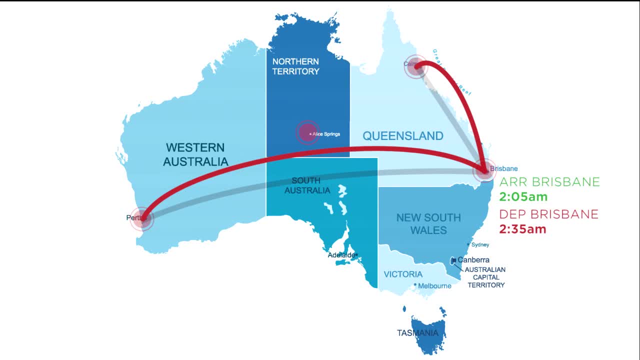 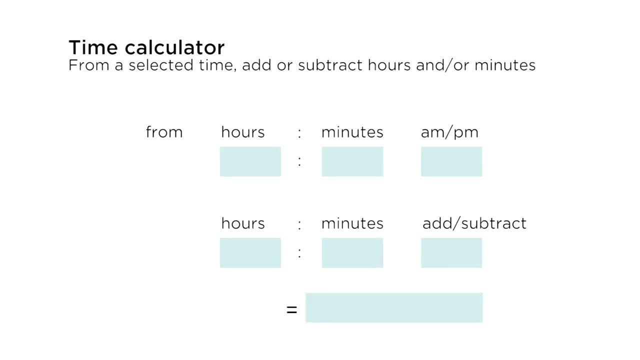 2 hours and 20 minutes. She's then got a 30-minute wait for her connecting flight in Brisbane to travel to Perth, which takes 4 hours and 59 minutes. What will be the time in Perth when she lands? Her departure time is 2.35am. 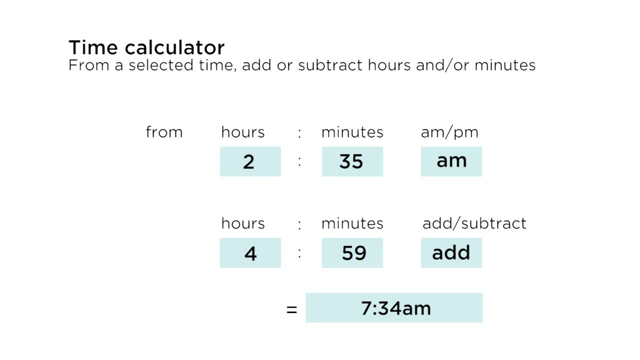 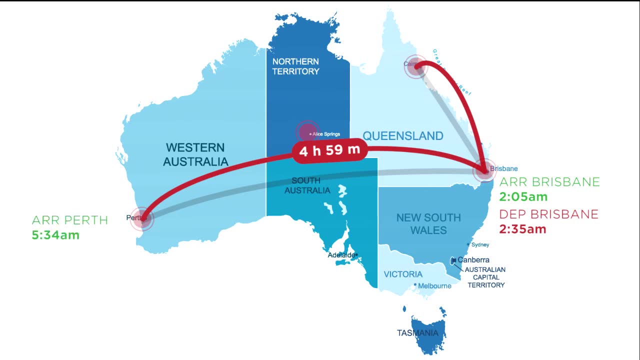 So it's 7.34am But Perth is 2 hours behind, so local time there will be 5.34am From Perth. she's going to Alice Springs, flying out at 10.15am and landing in Alice Springs at 2.44pm. 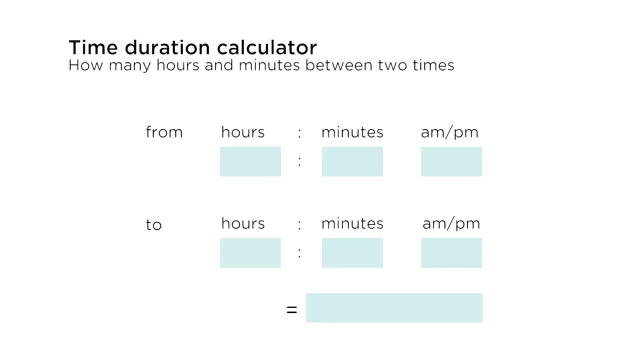 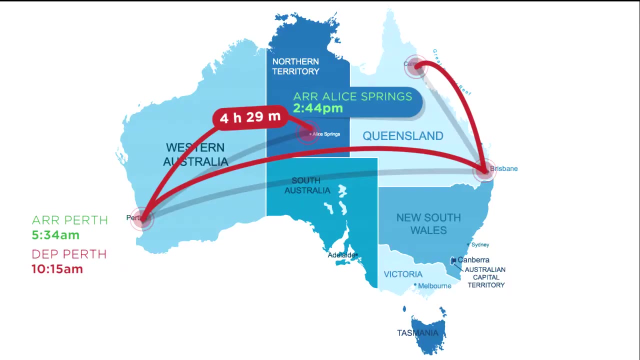 So how long is that flight? Using the time calculator, 4 hours and 29 minutes is the answer it gives. That seems like a long flight. That's because Alice Springs' time is an hour and a half ahead of Perth, So I have to subtract an hour and a half. 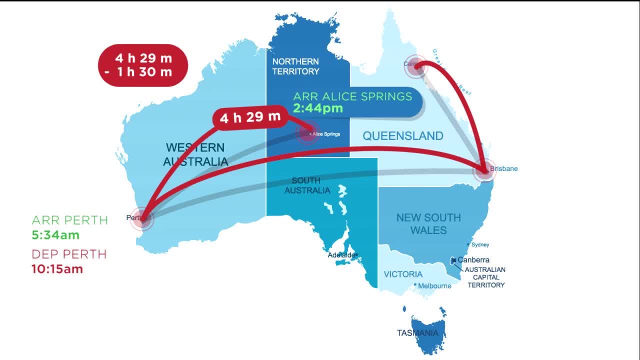 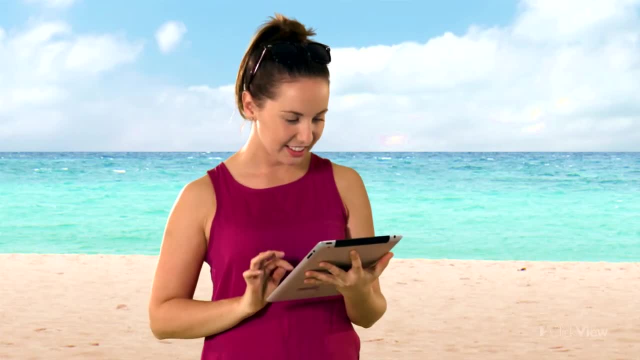 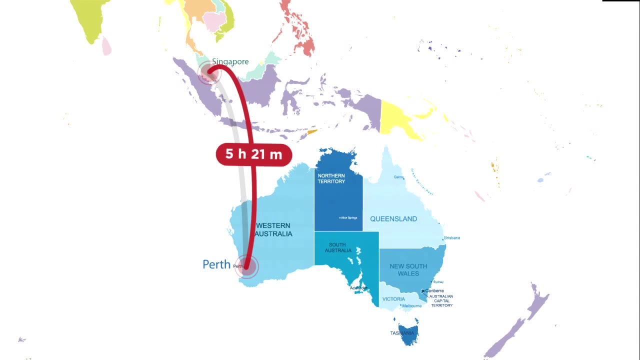 from the flight time, It actually only takes her 2 hours and 59 minutes for the flight. She returns to Perth for a week and then she flies back to Japan via Singapore. The flight to Singapore takes 5 hours and 21 minutes. 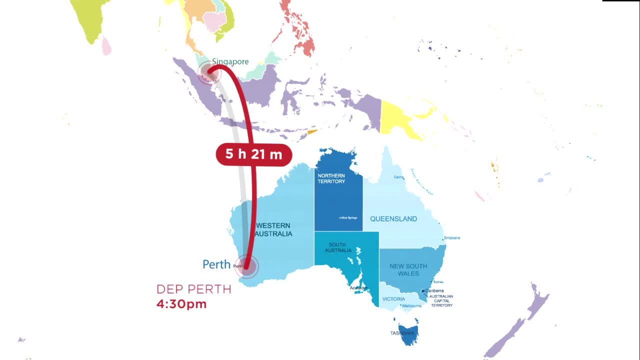 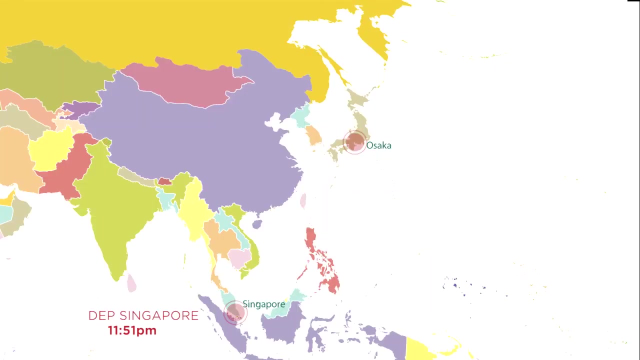 Departure time from Perth is 4.30pm, So what time will she land in Singapore? 9.51am, And they're in the same time zone, so no adjustment needed. A two-hour wait at Singapore before flying back to Osaka.